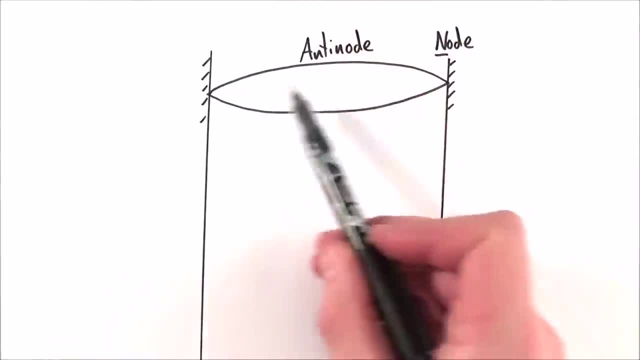 And all I've drawn in here is effectively the maximum and the minimum position of perhaps, a string which is vibrating. I can repeat it for perhaps the second kind of standing wave that we can fit in. So again, we're going to have a. 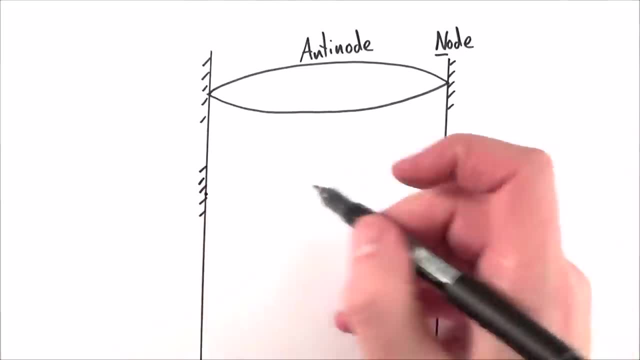 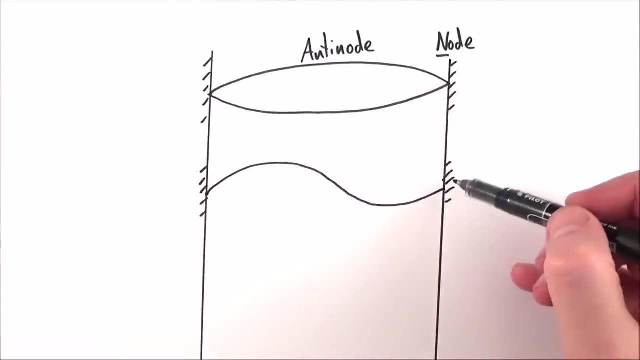 The ends must be constrained. but this time there's another wave that is actually the length of one complete wavelength And if I draw that as one of its waveforms, the opposite to this at the other extreme, half a cycle later, looks a bit like this: 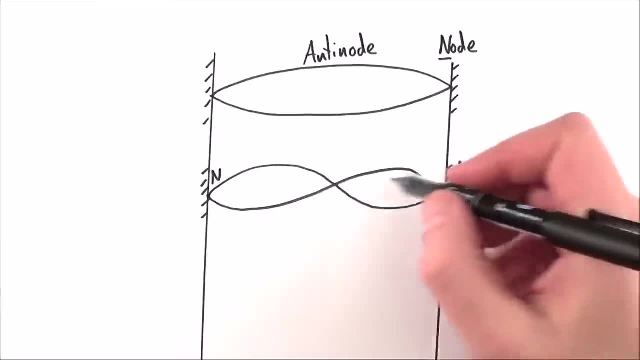 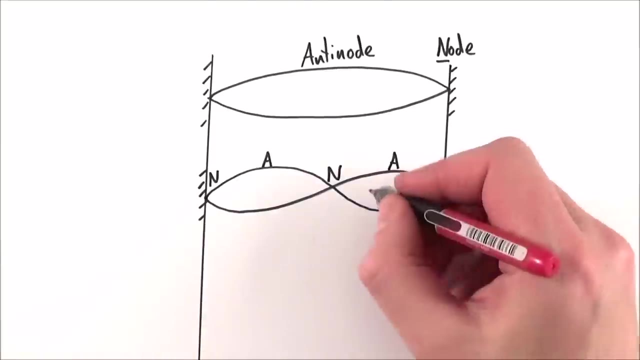 And again we have a node at each end. We also have a node or a point of no displacement in the middle, and then we have an antinode and another antinode. Now the key thing about this Is that, because this is one wavelength, the distance from a node to another antinode is equal to the wavelength of that wave over two. 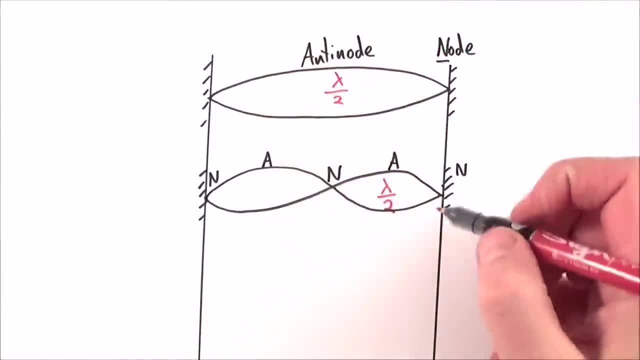 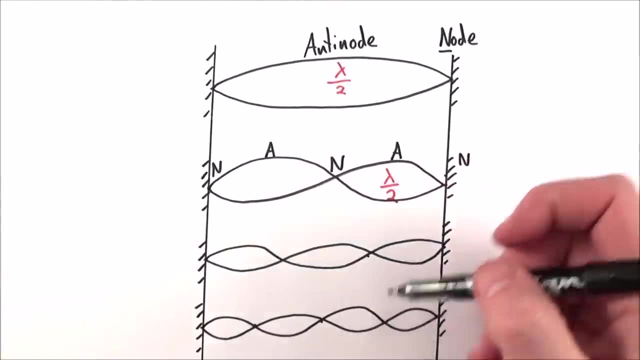 And this one here. this is also equal to the wavelength over two, and so on, And if we repeat the process, what we have here, although slightly dodgily drawn, we do have various other standing waves that can be set up within the same distance. 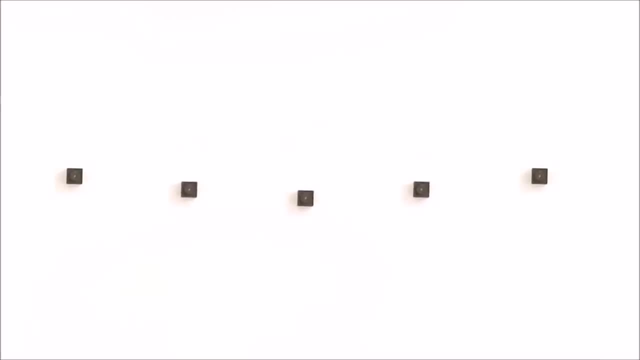 From the diagram so far, they all look a bit static, so this is what it would look like. Here we have a couple of nodes and the particles moving up and down in the middle, And then we also have another wave that has three nodes and also one that has four. 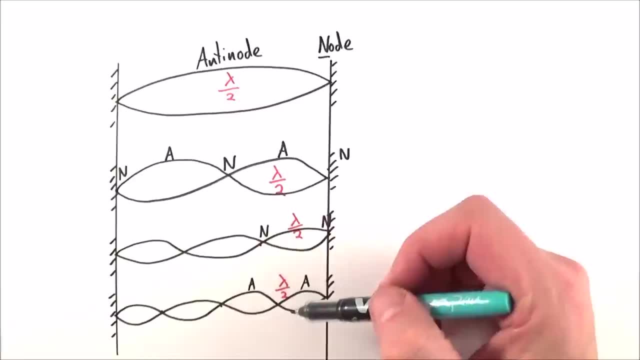 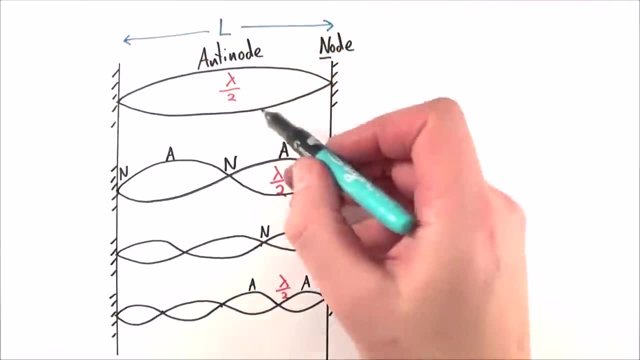 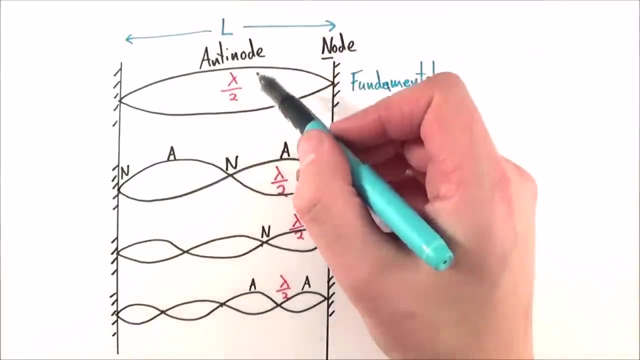 Looking in a bit more detail at these various diagrams here perhaps we have a string that has length L, And what we have here is the first standing wave that we can produce What we call. this is the fundamental For this fundamental, because the length is equal to the wavelength over two. 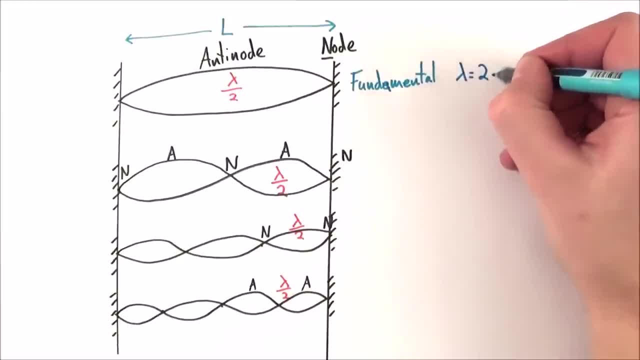 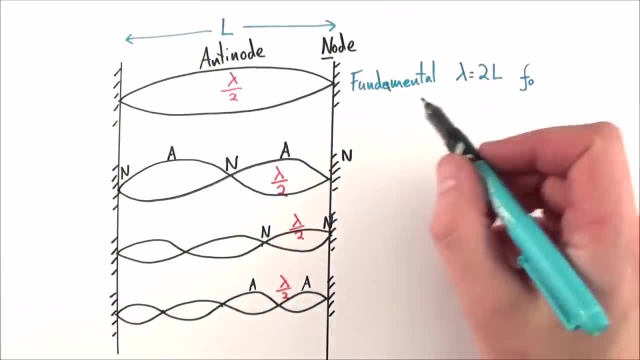 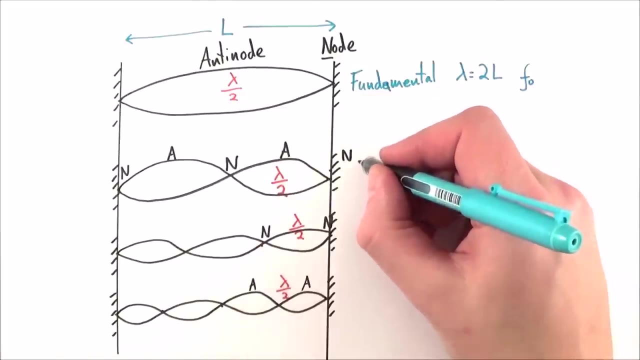 we can say that the wavelength is equal to two L, And this happens at a certain frequency, which we call F naught or F zero, And that is the fundamental frequency of that standing wave. Now there's another one here. This time, what we call this is the second harmonic.